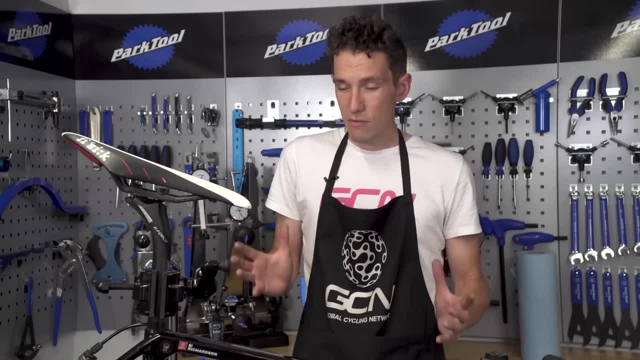 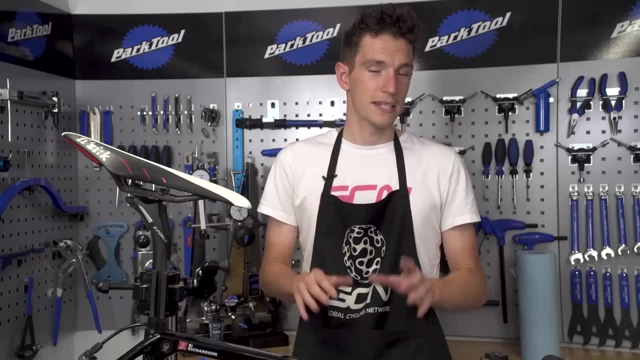 that is, via a galvanic reaction, You can generally remove stuck seat posts. We've actually got a video showing you just how, but I'll warn you, you will probably need to sacrifice your seat post in order to do it. So, rather than 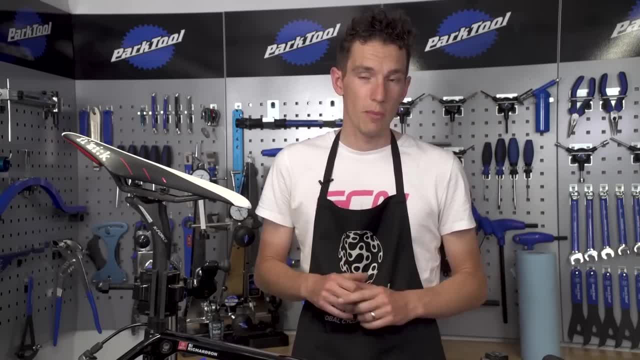 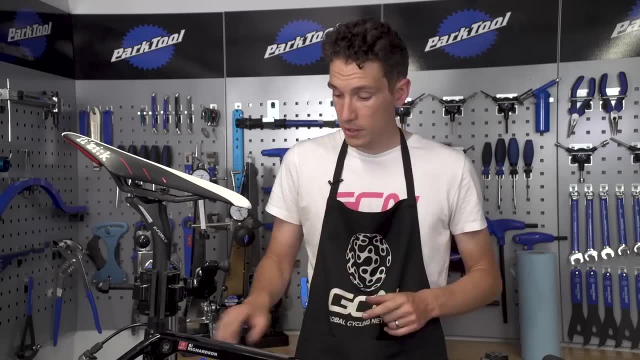 go through all that irritation and expense. do one simple job, and that is remove your seat post, put a layer of grease on it before putting it back into place, And, if it's a carbon post, into a carbon frame. you want to try using a fibre grip product instead. 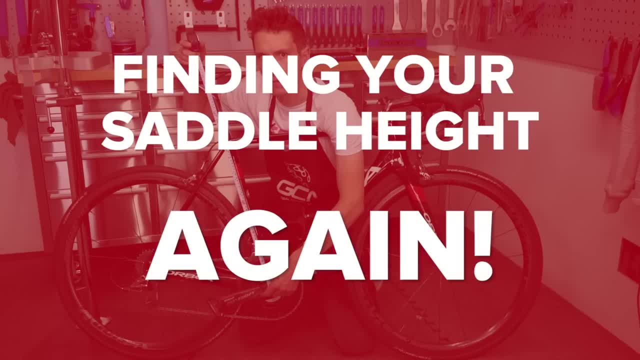 Getting the right saddle height again. Now, this is going to be a bit of a challenge, but I'm going to give it a try. I'm going to try to get it to the right position Now. this one might bother some of you more than others, but it definitely bugs me If. 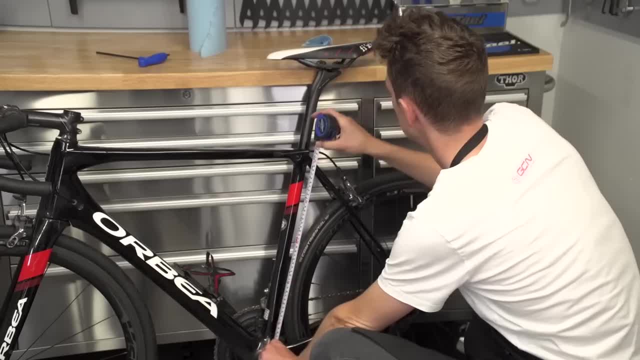 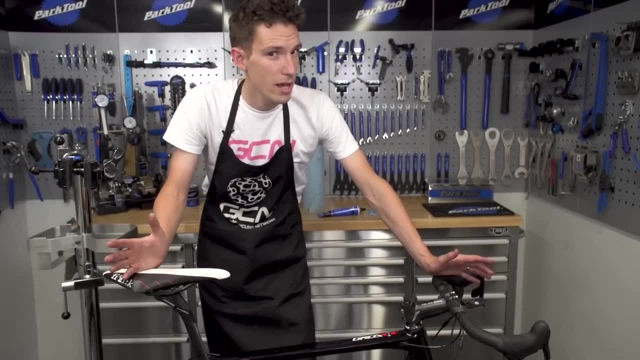 you ever need to remove your seat post for any reason, then getting it back in exactly the right place can drive you nuts. You're out riding and it feels fractionally too high or it feels fractionally too low, And no matter how many times you move it no matter. 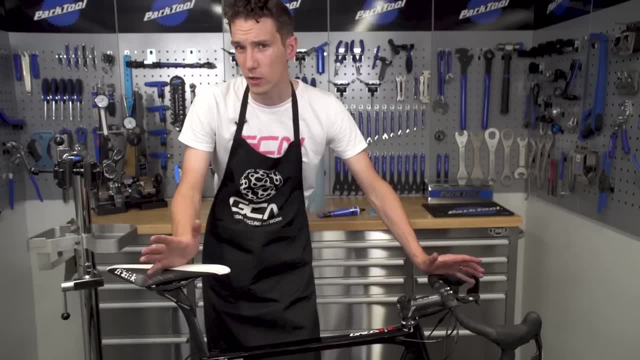 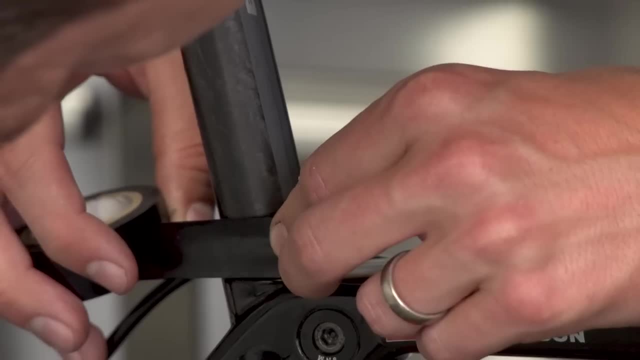 how many times you measure it, it still feels wrong. But there is a quick fix. All you got to do is put a piece of electrical tape around your seat post and you're good to go Just where it touches the frame. That way, no matter how many times you remove the post. 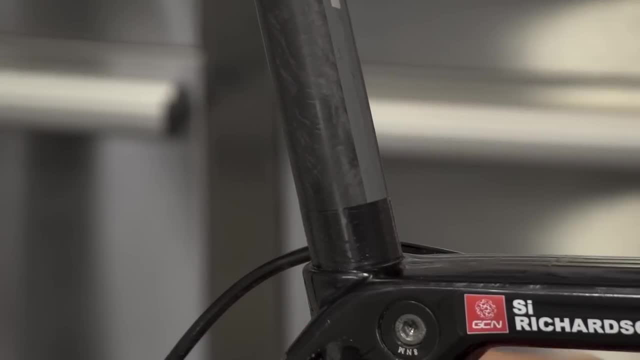 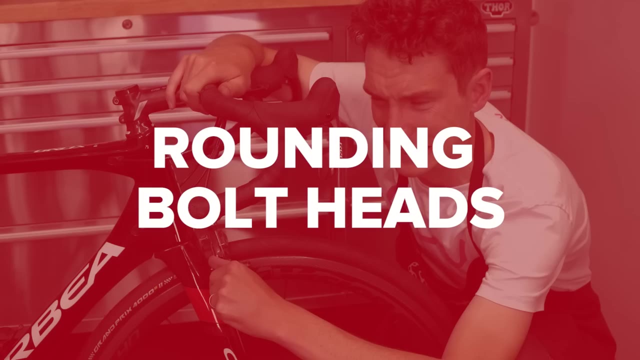 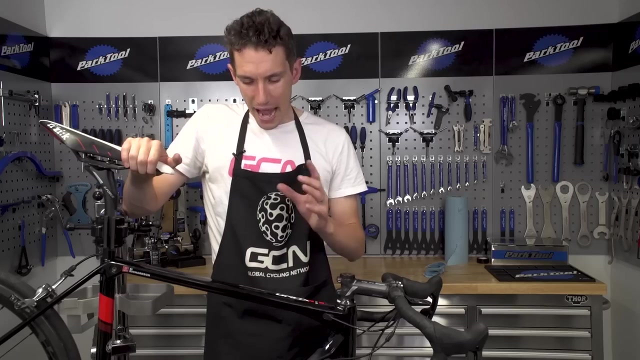 to make sure that it's not seizing. obviously, you'll know that it always goes back in exactly the right place. Rounding bolt heads, Stripping bolts so that you can't get them out, can be really, really annoying and lead to hours of faffing around trying to remove them, if it was even possible in the first. 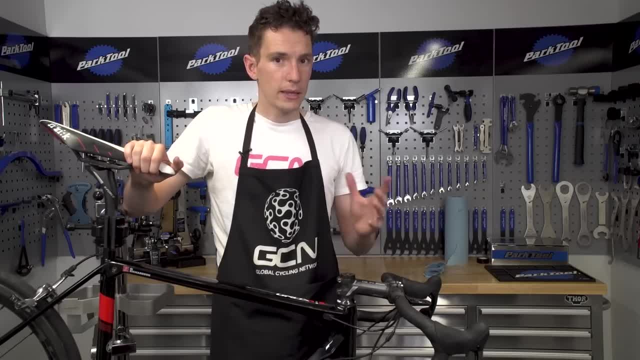 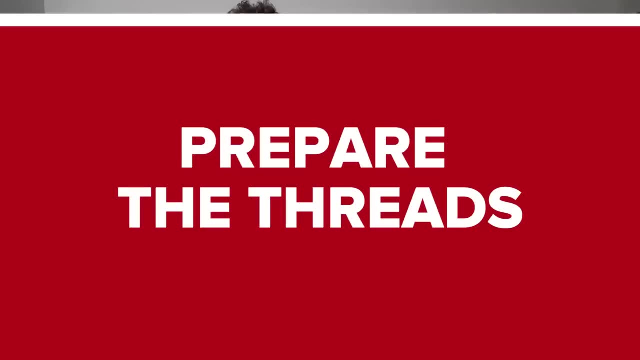 place. Obviously, sometimes there's nothing you can do about it. They just get stripped, But most of the time it's preventable. To do it, we need a two-pronged attack. Firstly, we need to prepare the threads of the bolt to make sure that we can actually 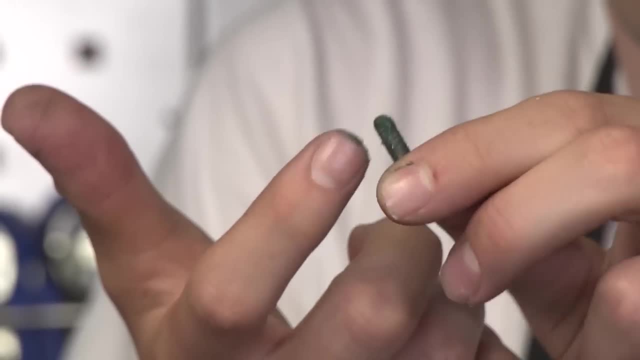 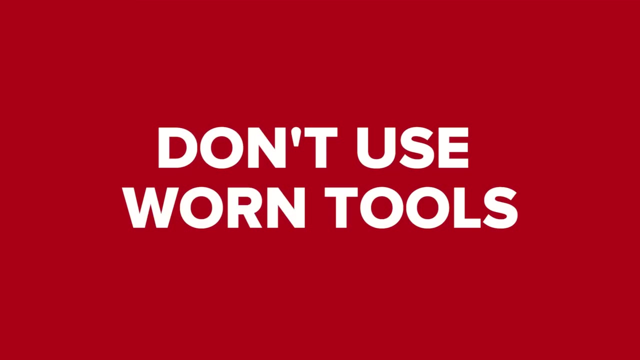 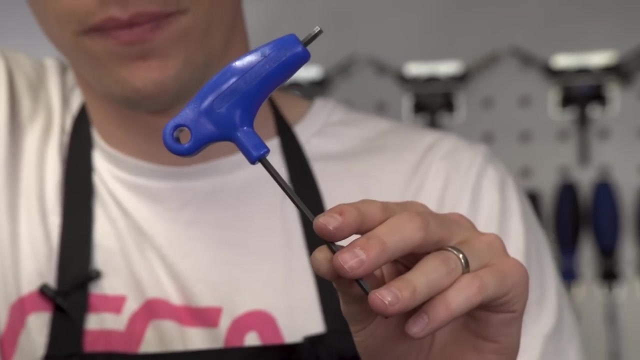 undo it when we need to. So it might be just a layer of grease, It might be a thread-locking compound, But either way, most bolts will need some kind of prep. Secondly, when it then comes to Either tightening or loosening your bolts, use a good quality tool, And remember that. 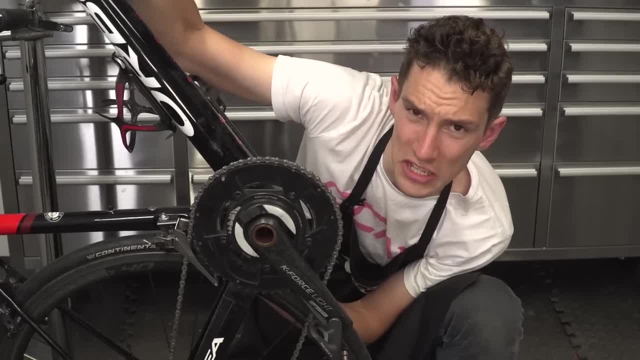 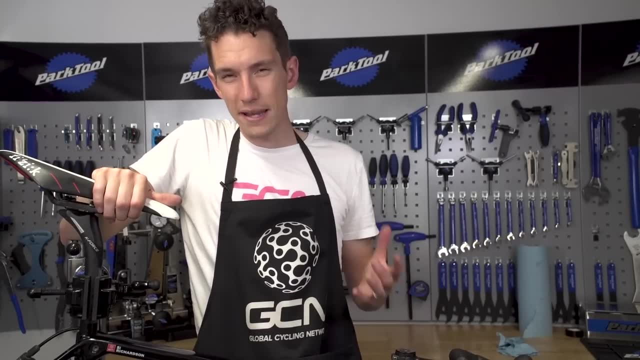 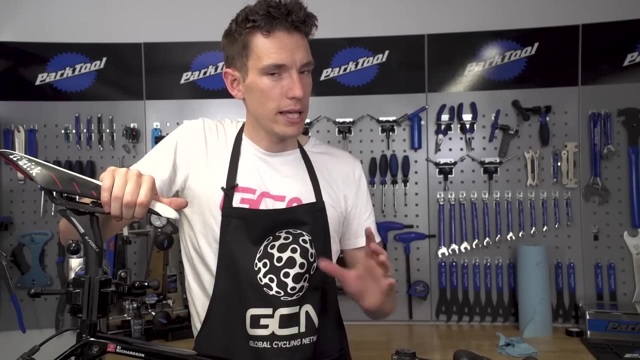 worn tools, wear bolts, Lost internal cables. Internal cables are cropping up on more and more bikes and at lower and lower price points, which is great because they look super cool. However, if you're not careful, they can actually drive you insane. 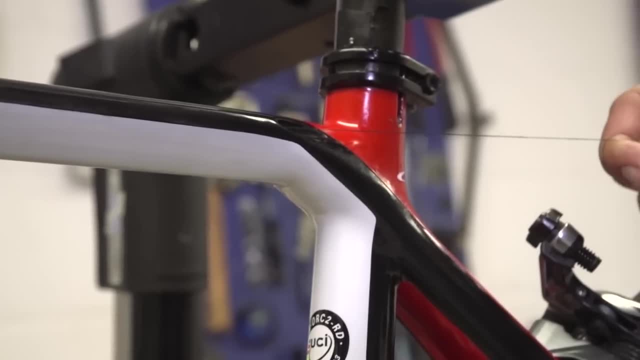 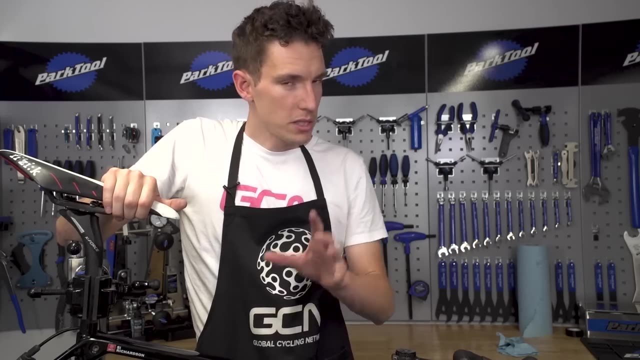 If you remove a cable without taking steps to handle it, you're going to lose a lot of weight, And if you don't help to re-thread it before you do so, then you could end up losing hours off your life. So consider this a timely reminder before you do it, When you go to remove a cable. 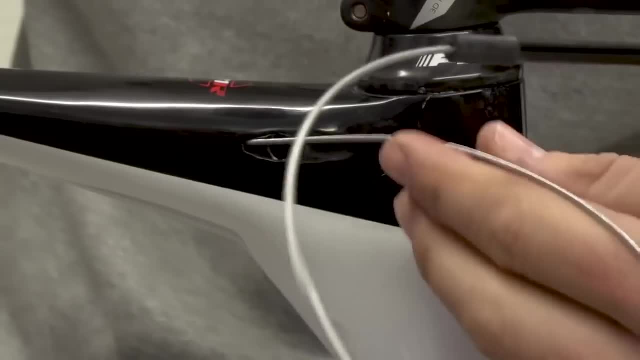 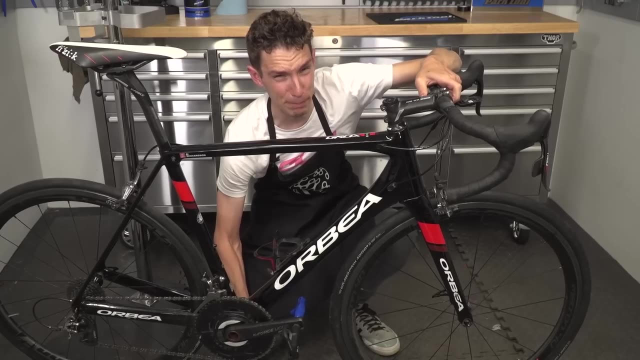 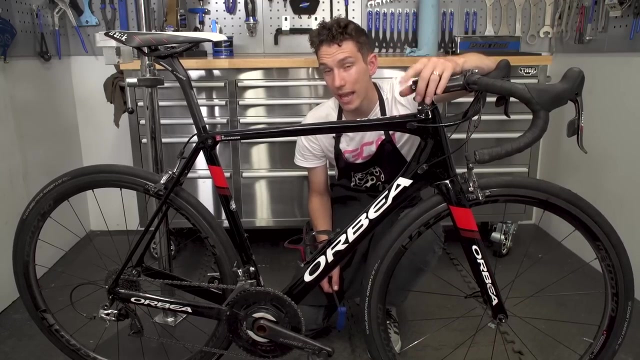 take a little tube, thread it over it through the frame so that when you then finally remove the cable, the tube is left in place as a guide. to help with the next one: Stuck pedals. Taking your pedals off can be surprisingly annoying. 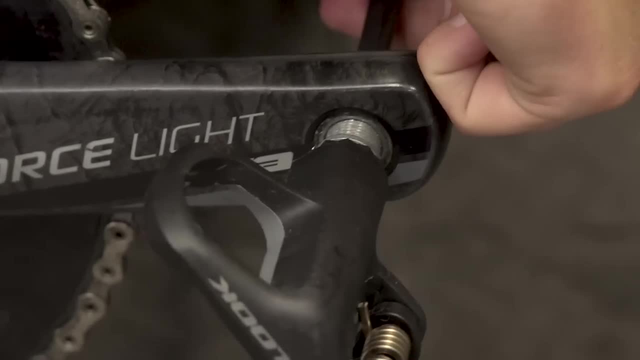 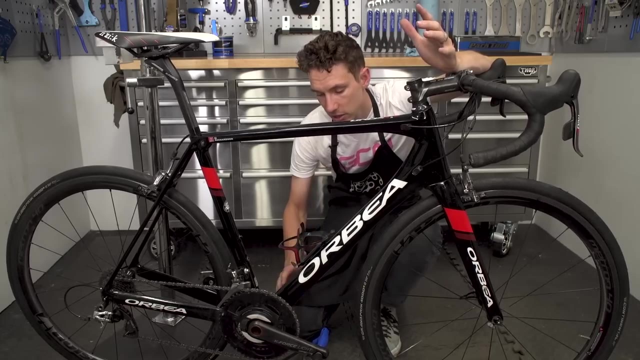 And surprisingly painful as well if you're not careful. Mainly it's just technique based, so take a little bit of time before actually taking them off to make sure the allen key or the wrench is in a position that you're not going to skin your knuckles when it suddenly loosens. 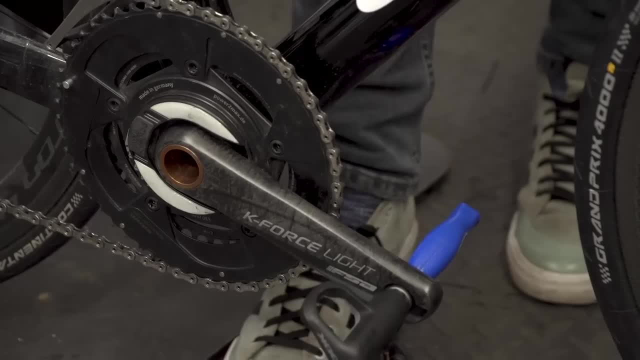 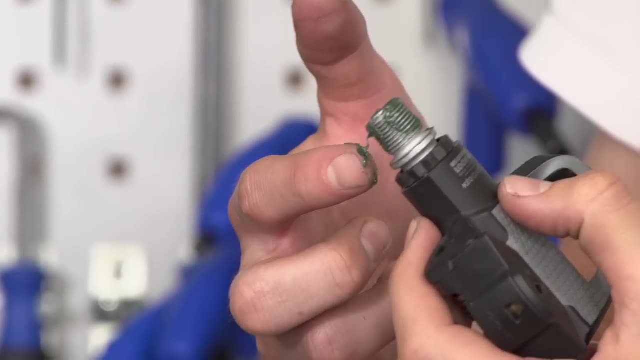 And if the pedals are on too tight, consider getting your foot involved as well. But then, harking back to our previous point, make sure that you grease the threads of your pedal axles before you put them in in the first place. That way you're going to avoid. 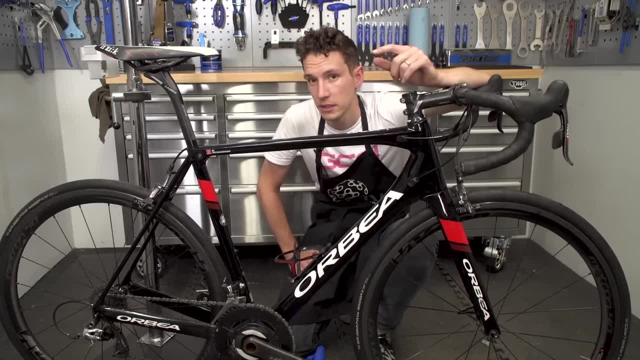 having them seize into your cranks. And also you're going to want to make sure that your pedals are in the right position. If you're not, then you're going to want to make sure that you don't over tighten them. 35 newton metres will do the trick if you've got a torque wrench. 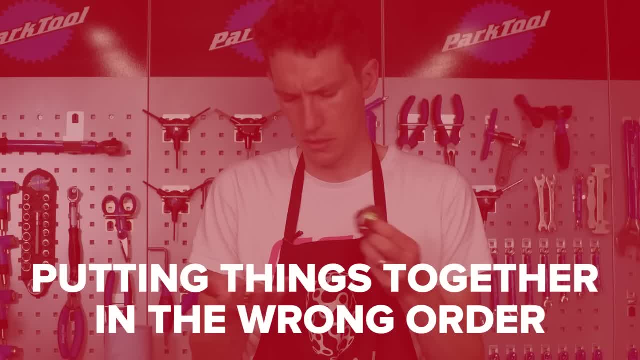 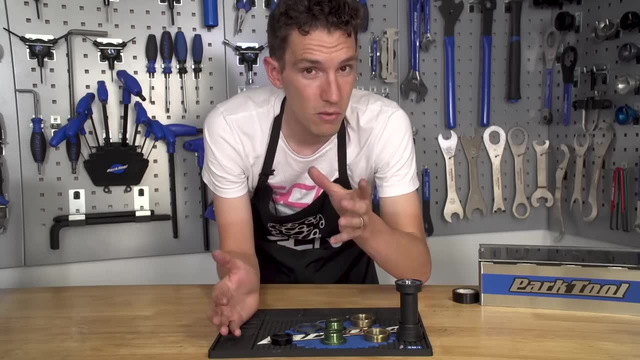 Putting things together in the wrong order. Most bike maintenance jobs are relatively straightforward. You can take things apart and put them back together again relatively simply. But there are a few jobs that are more complicated. Now. I'm thinking mainly bottom brackets here, but also headsets to. 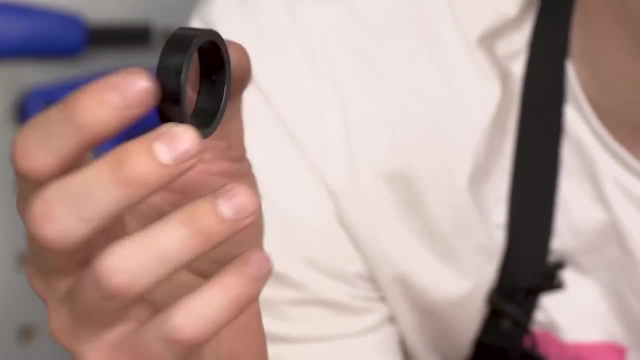 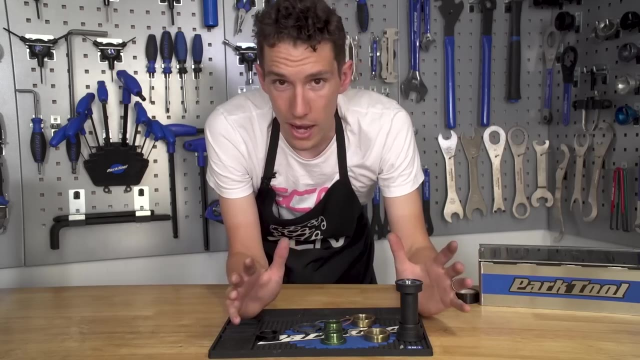 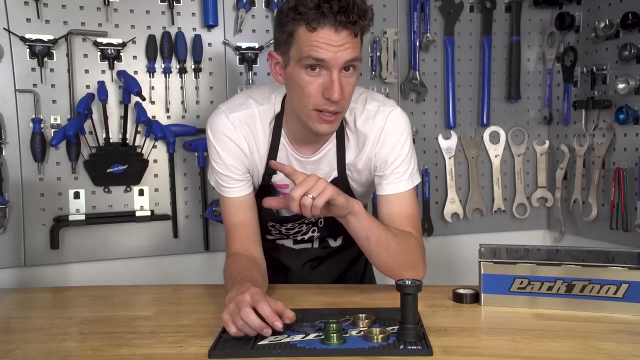 a certain extent. What spacer goes where, and where on earth did that flippin' seal come from? Queue hours spent trying different permutations, even when you have the instructions in front of you. Now, it's not exactly a hack, this, but it is definitely a timely reminder that 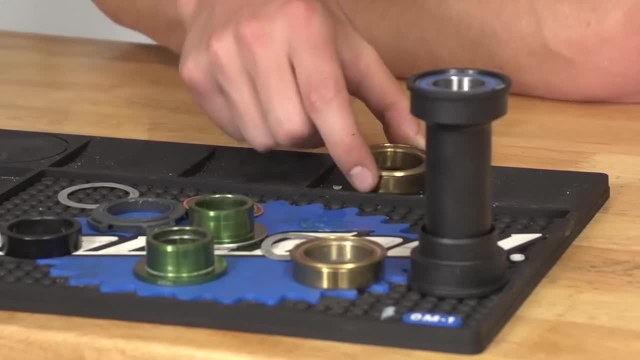 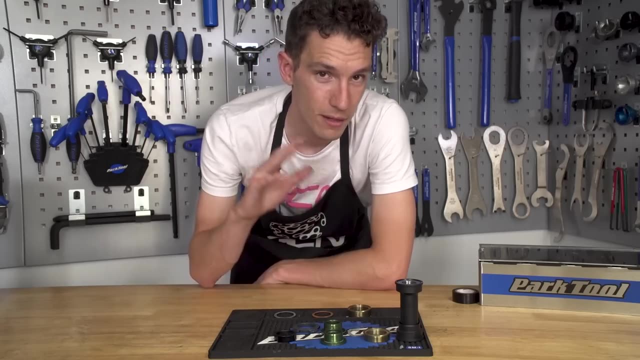 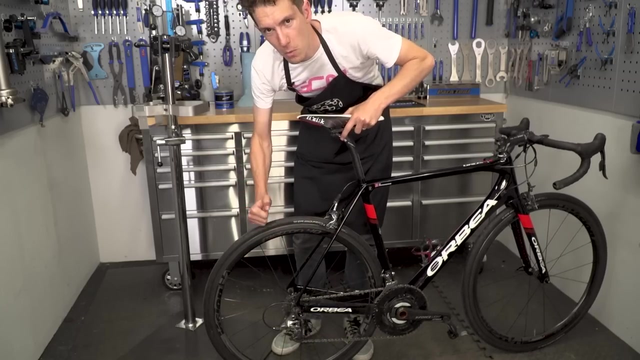 if you just spend 10 seconds keeping a track of how things come apart, either taking photos or literally just lining them up on your worktop, then you will be able to put things back together again very simply and save yourself a lot of time Not being able to get your back wheel. 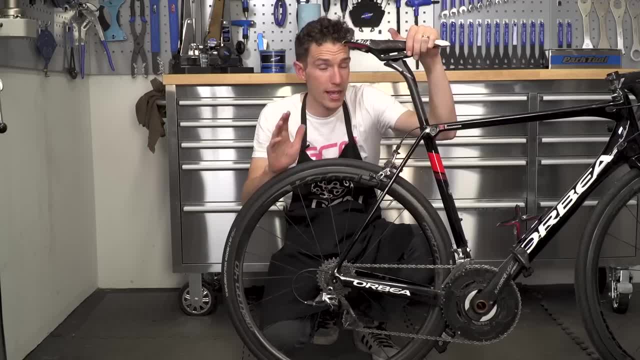 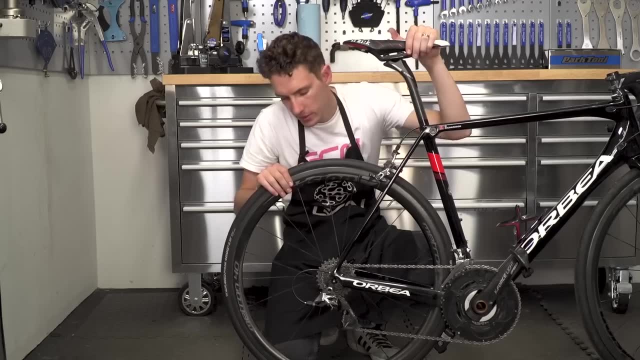 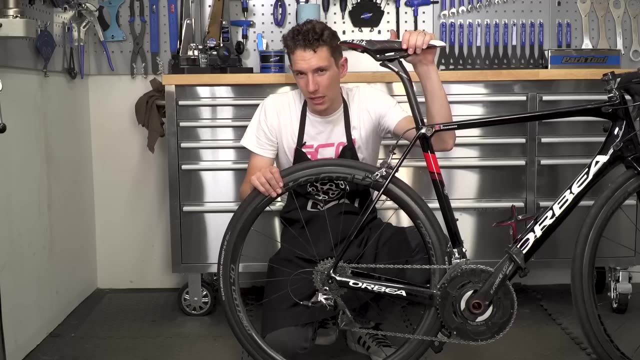 out. Here is a simple one, but I'm sure we're all guilty of it, Or at least I know I'm guilty of it. You need to take your back wheel out and you know that you need to put your chain in the smallest cog on your cassette, But you just can't really be bothered, I mean. 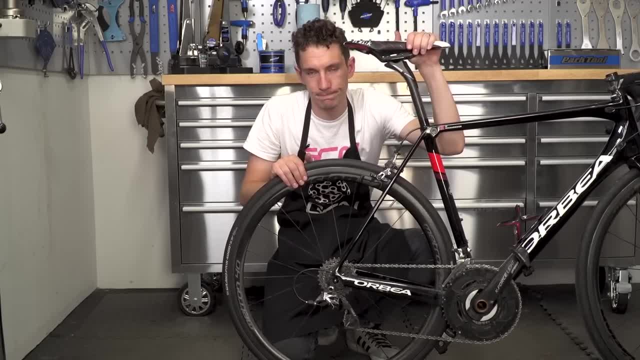 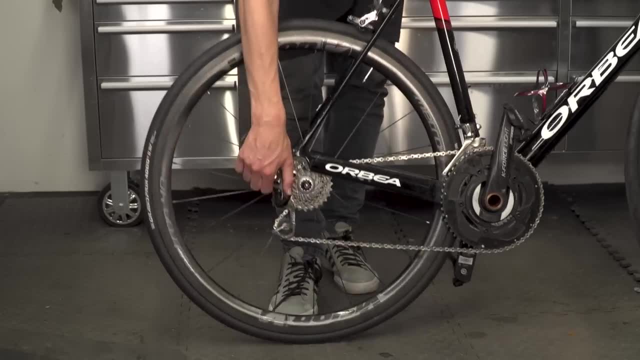 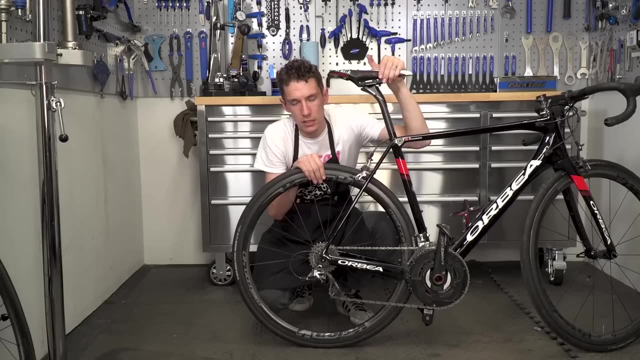 how much harder is it going to be to get your back wheel out? A lot harder, In fact, much, much, much harder. So, rather than try spending ages faffing around getting your back wheel out with your derailleur in the wrong position, 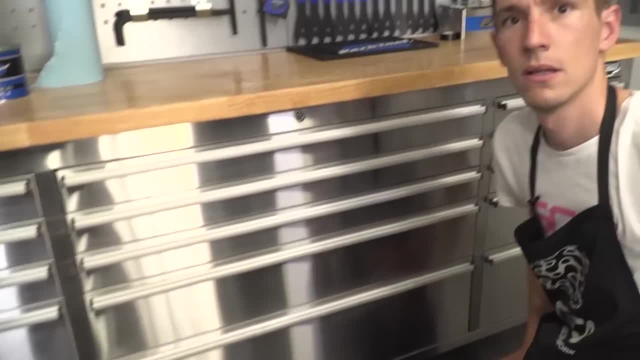 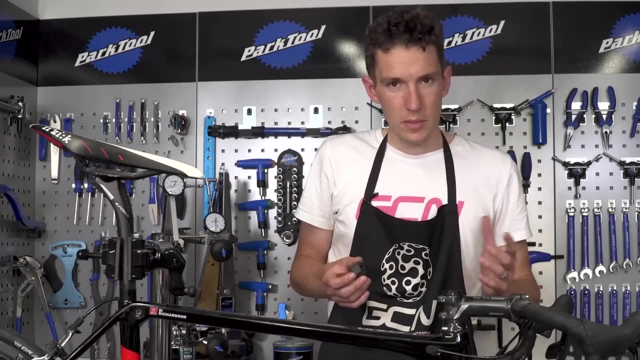 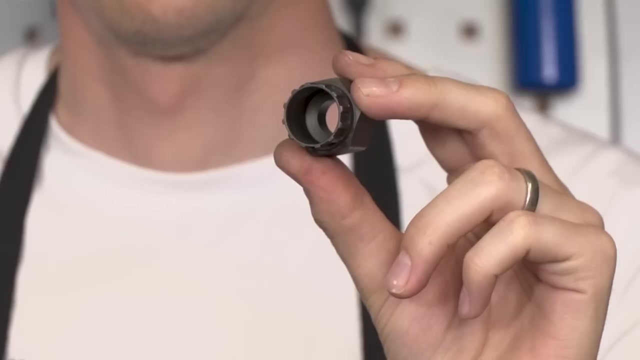 just change gear. first Searching for tools. Now, this used to be another one of my specialities: Losing tools. Man, the amount of time I lost one winter trying to find my cassette tool- And it wasn't a one-off either, It was a regular. 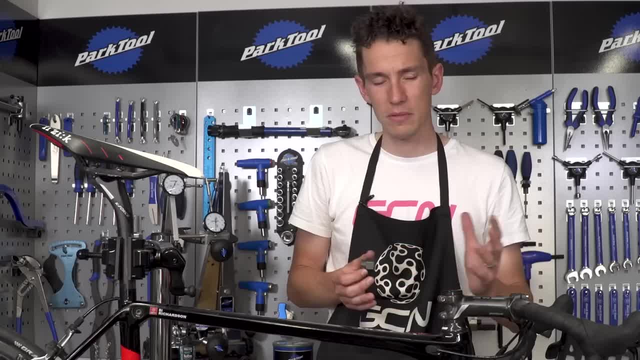 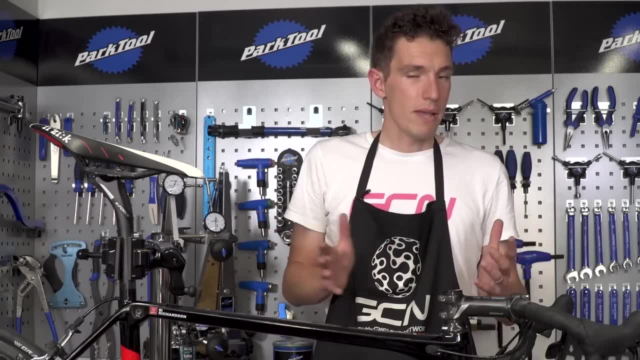 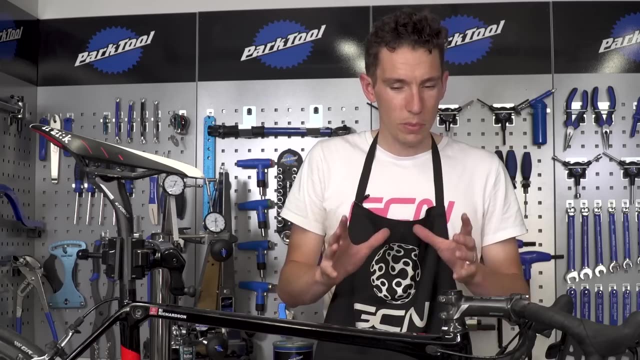 thing Still happens from time to time now, as I absentmindedly put a tool down somewhere random and then completely forget all about it. Now, of course, this isn't a maintenance job, but it is nevertheless a mind-blowingly irritating thing and easy to prevent as well. Just create a special place to keep all your bike maintenance. 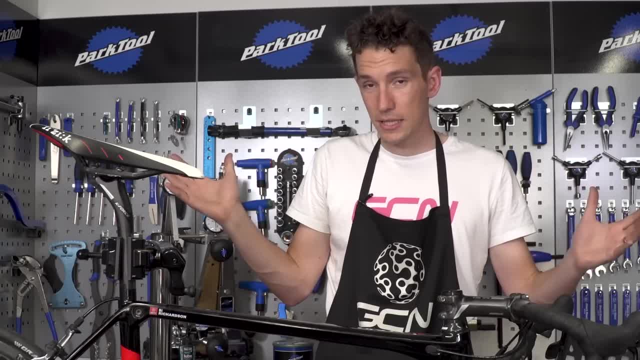 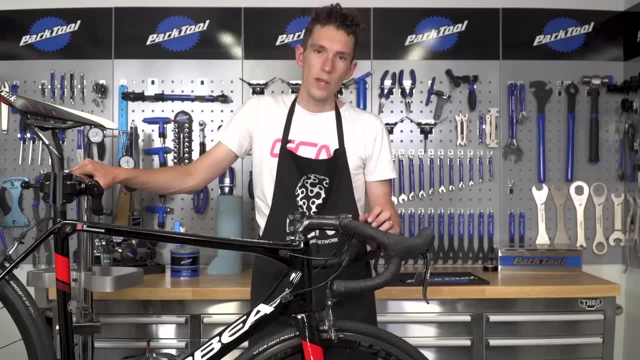 tools. We're not, of course, all going to be as lucky as this, but a small tool box or a small tool wall will make working on your bike that much quicker and that much easier, With the exception of helping to look for lost tools, which we haven't covered on the channel yet, although 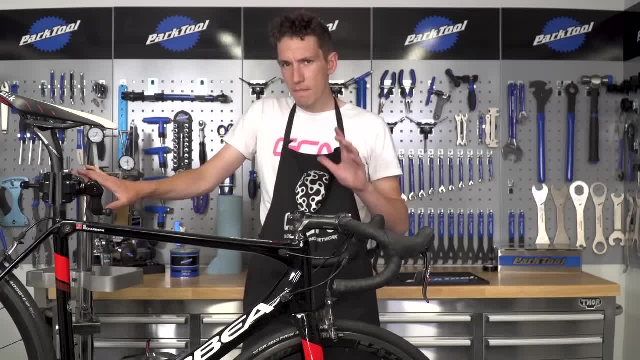 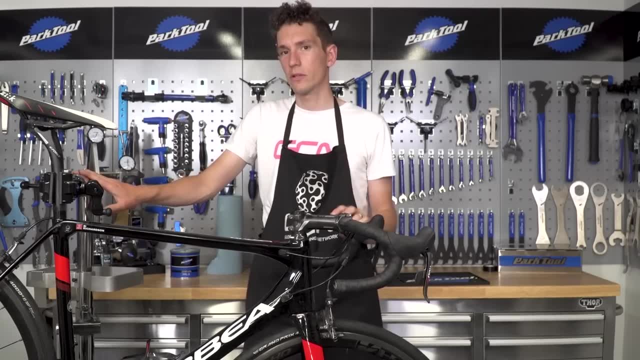 that is actually quite a good idea. we've got videos about most of the unfortunate outcomes talked about in this video. How to remove stripped bolts is in fact coming soon, so do make sure you subscribe to GCN by clicking on the globe to make sure you don't miss that one. And then for a couple. 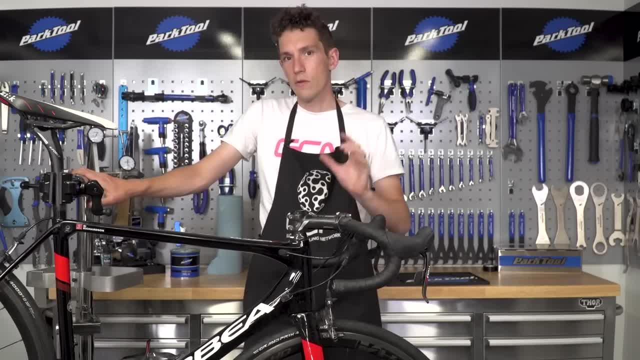 more. why not click just down there to help remove a stuck seat post, if you need that, Or indeed down there for help with internal cable routing? Thanks for watching. We'll see you next time.